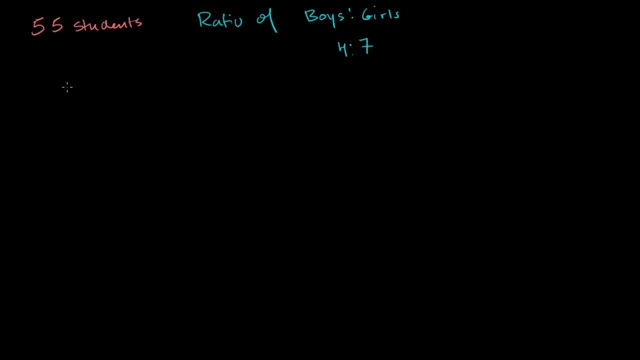 What I want to know is: how many girls do I need to add? So, how many girls do I need to add for the ratio to become 1 to 2? 1 to 2.. 2 to 2. And this is the ratio of boys to girls. 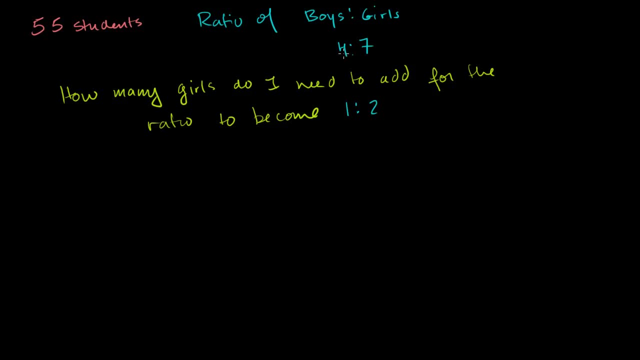 I'm not switching the ratio on you. So right now, for every 4 boys, I have 7 girls. I want to add some girls so that the ratio becomes: for every boy I have 2 girls. So how can we do this? 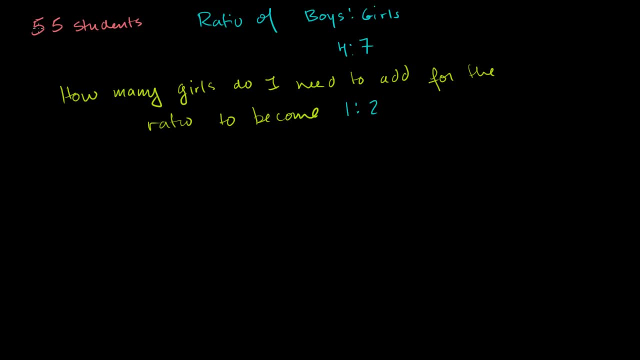 Well, just going back to the basic ratio video, the first thing we can do- we know the total number of students And we know the ratio, So maybe it'll help us to figure out the number of boys and girls we have right now. 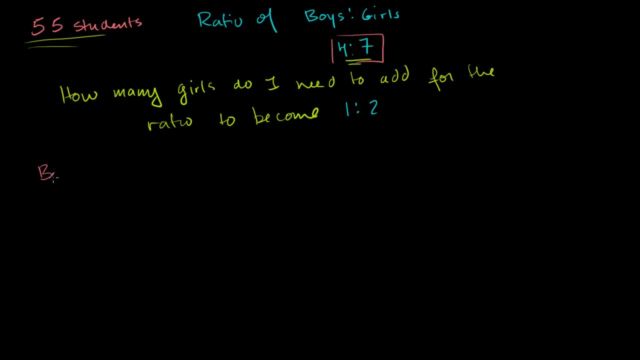 So our current ratio is 4 to 7.. So boys, Boys to girls right now is equal to 4 to 7.. That means what does that mean? That means for every: if you add up these two, for every 11. 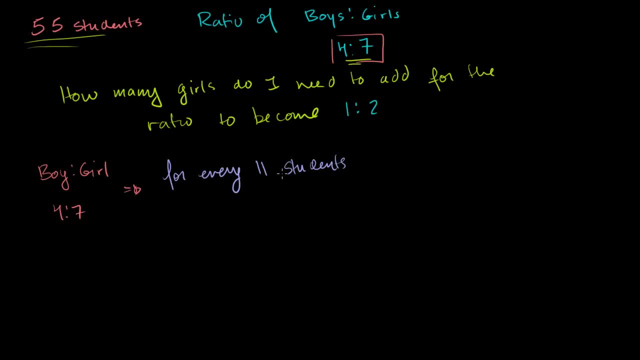 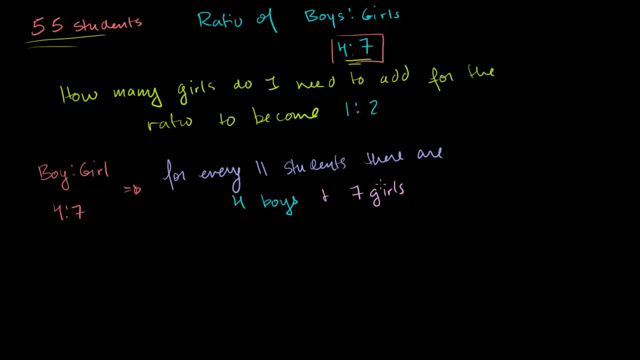 7 girls And 7 girls. That's what this ratio tells us. You give me 11 students of this. well, you could split this classroom into a bunch of groups and for every group of 11, you're going to have 4 boys and 7 girls. 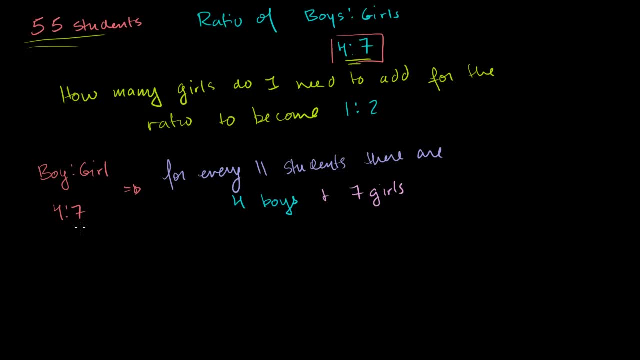 That's all that tells me For every 11 students: 4 boys and 7 girls. If you split them, I guess every group has the same number of boys and girls. Now how many groups of 11 students there are. 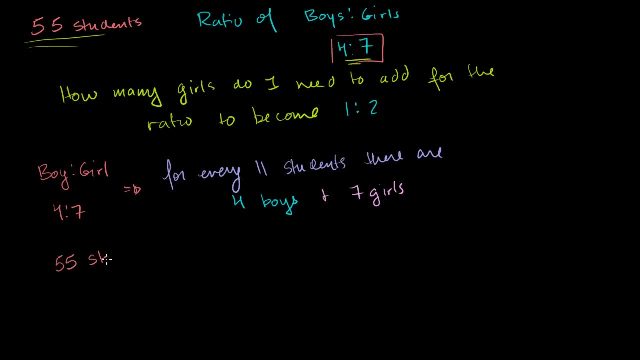 So there are 55 students. We have 55 students total And we're breaking them into groups of 11, and every group will have the same number of boys and of girls. So we have 11 groups, 11, sorry we have. we divide by: 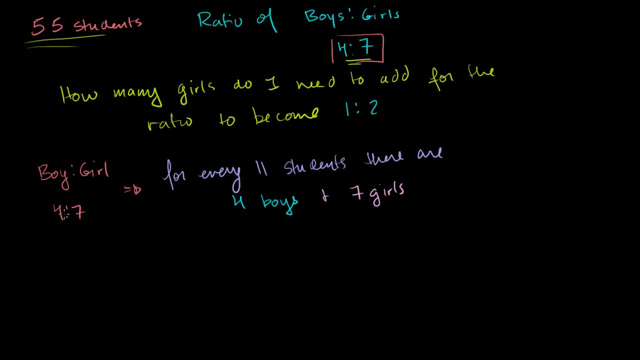 You give me 11 students of this. well, you could split this classroom into a bunch of groups And for every group of 11, you're going to have 4 boys and 7 girls. That's all that tells me For every 11 students: 4 boys and 7 girls. 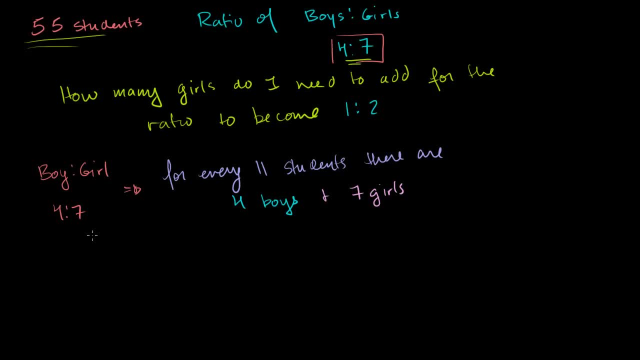 If you split them, I guess every group has the same number of boys and girls. Now how many groups of 11 students there are. So there are 55 students. We have 55 students total And we're breaking them into groups of 11.. 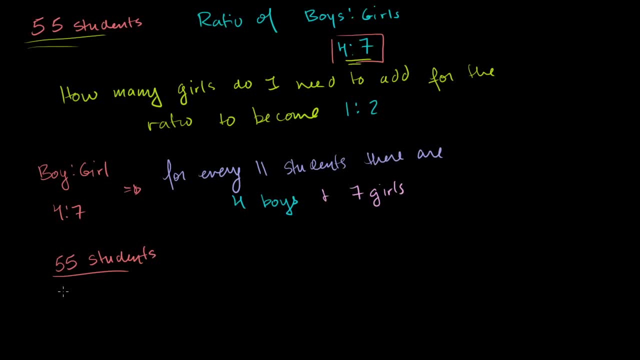 And every group will have the same number of boys and girls. So we have 11 groups. 11,, sorry, we have. we divide by 11. students per group, Students per group. So how many groups of 11 students do we have? 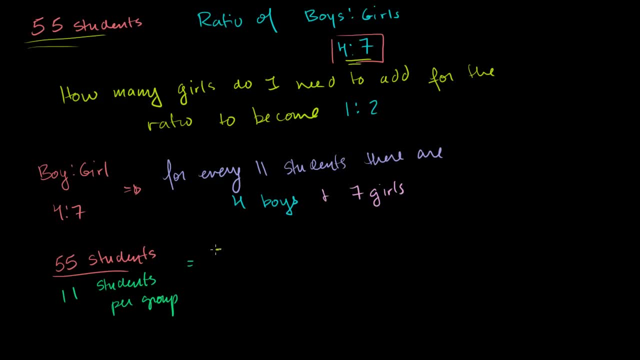 That means we have 5 groups of 11 students, 5 groups of 11 students. 5 groups of 11 students- And we've done this drill before- Every group has 4 boys and it has 7 girls, So we have 5 groups. 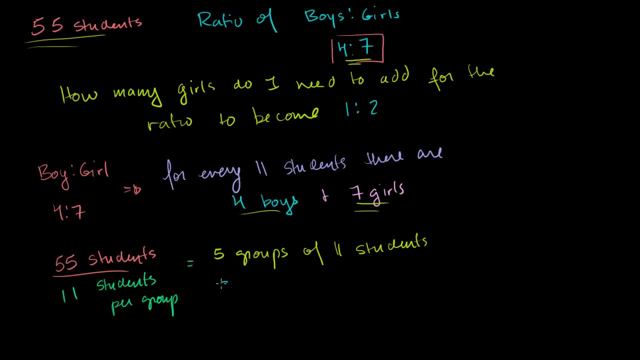 5 groups. each of them has 4 boys. That means we have 5 times 4, which is equal to 20 boys, And we have 5 times 7.. We have 5 groups 5 times 7.. 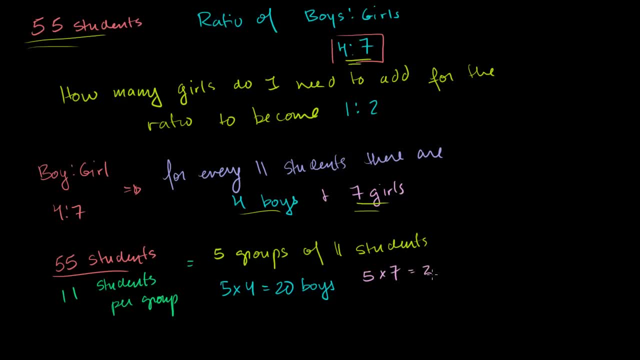 Each group has 7 girls Of girls, So that's equal to 35 girls. And the numbers add up, 20 plus 35 is 55. And 20 to 35 is equal to 4 to 7. So it all works out. 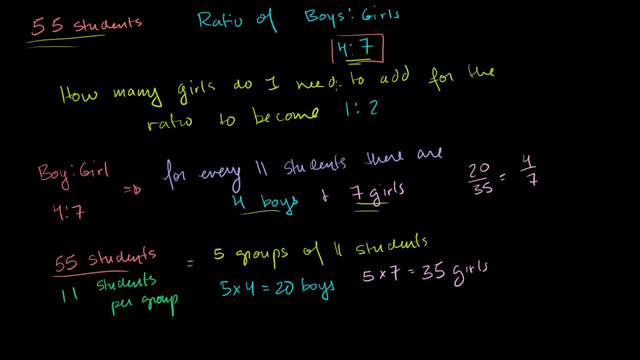 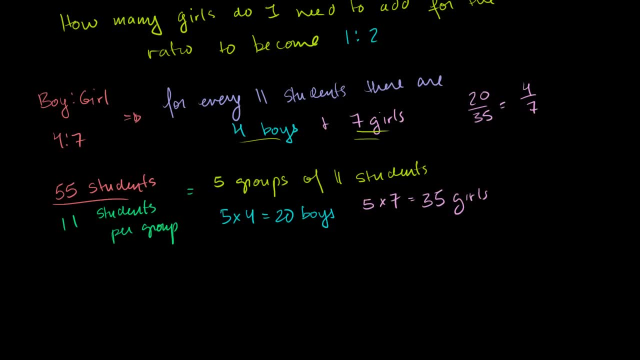 So that's what we have right now. Now we're going to add girls to the classroom to change the ratio, So let's do this. So right now we have 20 boys and we have 35 girls. We just figured that out. 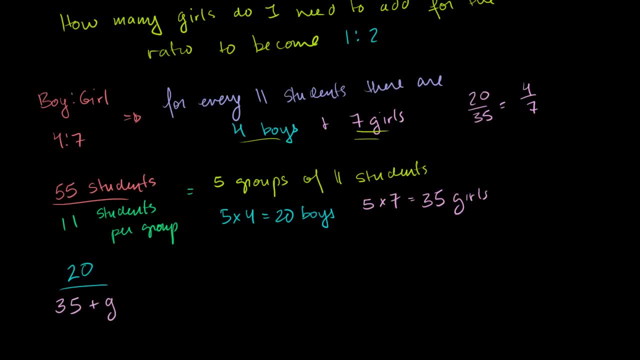 And I'm going to add some girls to the classroom. So I'm going to add some girls to the classroom And my new ratio, after I add these g girls to the classroom, my new ratio is going to be 1 to 2.. 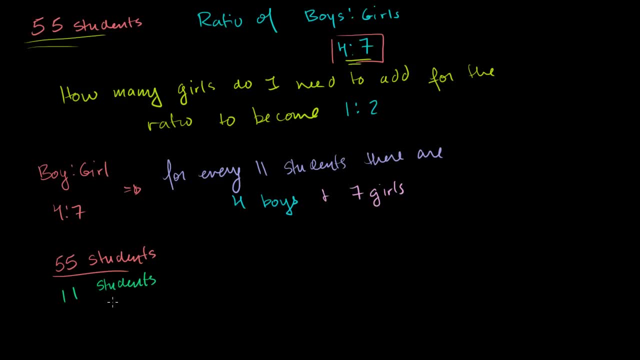 11 students per group. Students per group. So how many groups of 11 students do we have? That means we have 5 groups of 11 students: 5., 5., 5., 5., 5. 5.. 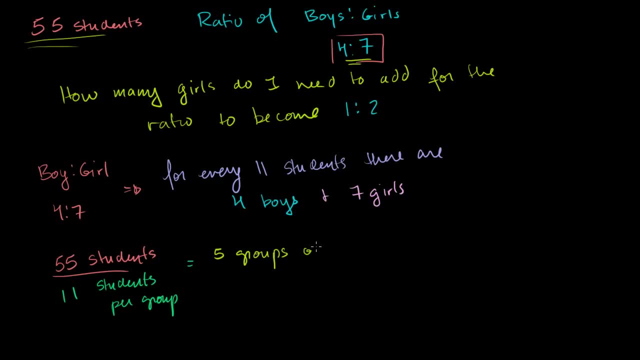 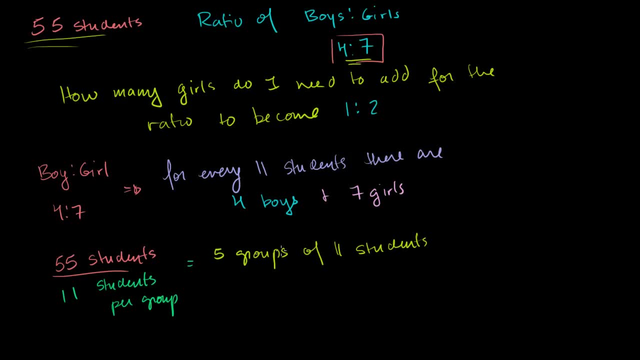 4., 5., 4., 6., 5., 4., 4., 4., 4., 5., 6., 1., 5. 1.. 11 students And we've done this drill before. 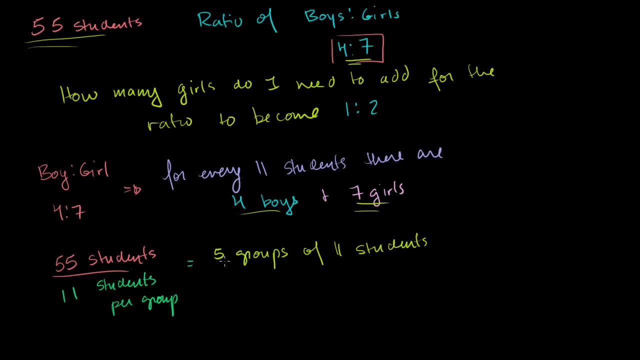 Every group has 4 boys and it has 7 girls. So we have 5 groups. Each of them has 4 boys. That means we have 5 times 4, which is equal to 20 boys, And we have 5 times 7.. 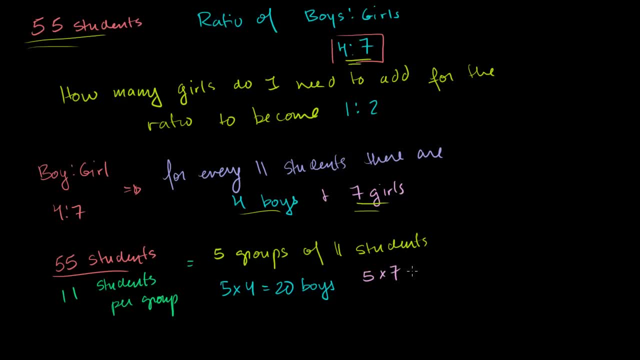 We have 5 groups, 5 times 7. Each group has 7 girls Of girls, So that's equal to 35 girls And the numbers add up 20 plus 35 is 55. And 20 to 35 is equal to 4 to 7.. 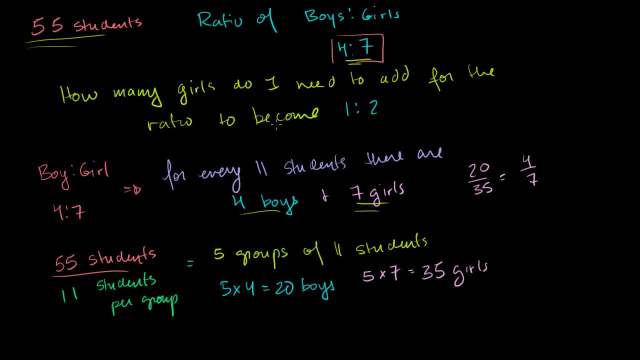 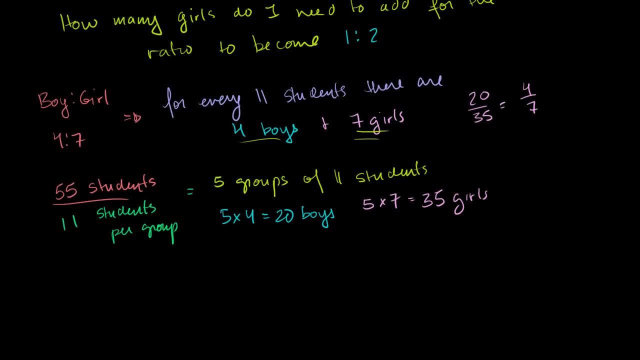 So it all works out. So that's what we have right now. Now we're going to add girls to the classroom to change the ratio, So let's do this. So right now we have 20 boys and we have 35 girls. 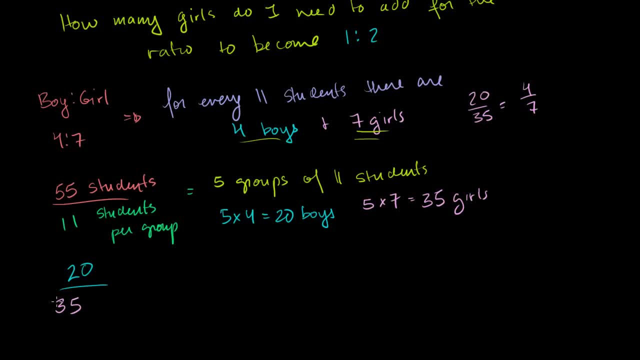 We just figured that out And I'm going to add some girls to the classroom. So I'm going to add some girls to the classroom And my new ratio, after I add these g girls to the classroom, my new ratio is going to be 1 to 2.. 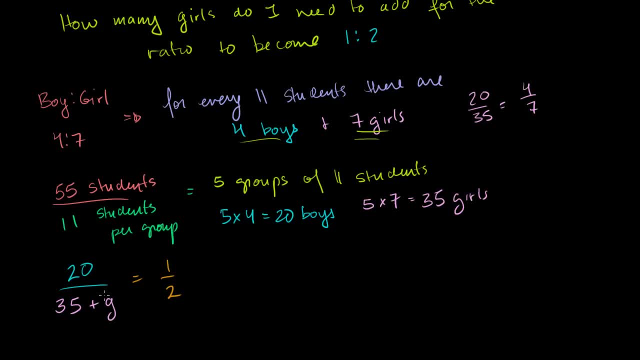 So I have an equation, I have one unknown. I can just solve for it. You can almost do this one in your head: 20 is to what 1 is to 2, as 20 is to what You could say. oh, 20 is. 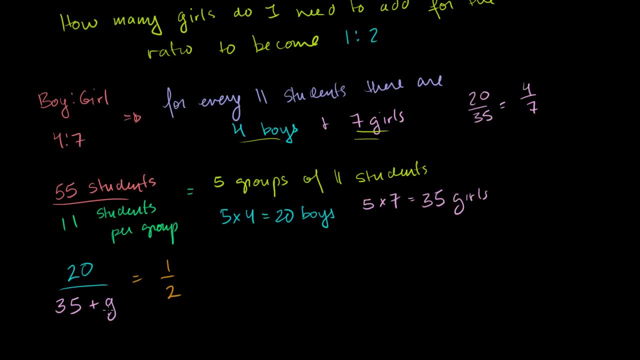 1 is half of 2.. 20 is half of 40. So you could say: oh, this must be 40. So g would be equal to 5.. That's how you would solve it in your head. If you want to do it algebraically, you could. 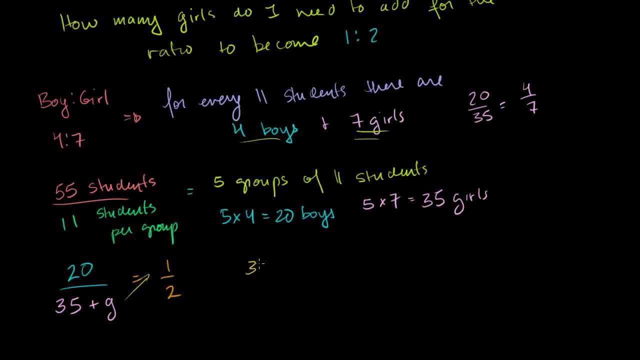 cross-multiply, So you get 35 plus g times 1.. So you get 35 plus g is equal to 2 times 20, is equal to 40, which is essentially what we did in our head. We said, hey, this thing has to be equal to 40.. 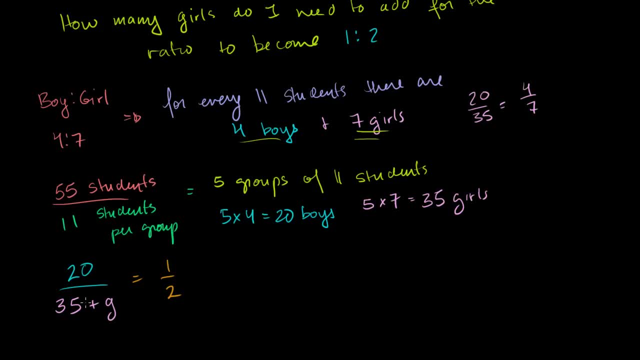 1 to 2.. So I just have an equation. I have 1, unknown. I can just solve for it. You can almost do this one in your head: 20 is to what, 1 is to 2, as 20 is to what. 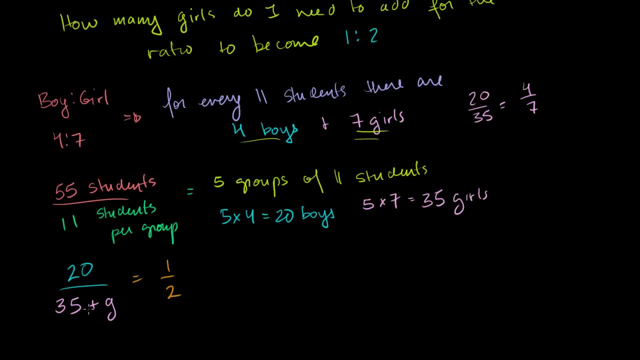 You could say, oh, 20 is, you know, 1 is half of 2.. 20 is half of 40. So you could say, oh, this must be 40. So g would be equal to 5.. 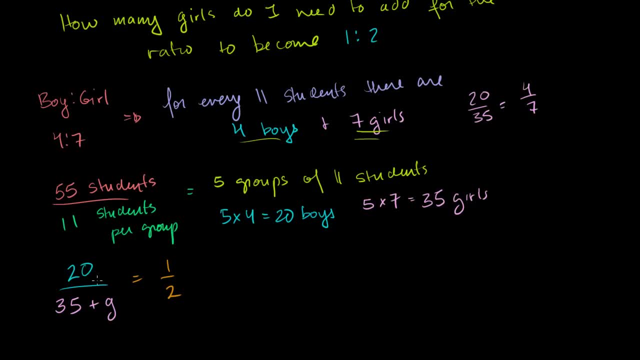 That's how you would solve it in your head. If you want to do it algebraically, you could cross-multiply. So you get 35 plus g times 1.. So you get 35 plus g is equal to 2 times 20 is equal to 40,. 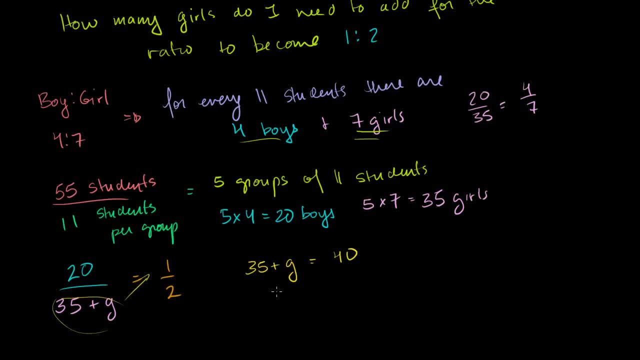 which is essentially what we did. in our head. We said: hey, this thing has to be equal to 40. So if you subtract 35 from both sides, you get g is equal to 5.. So if you add 5 girls to your classroom, you're going to 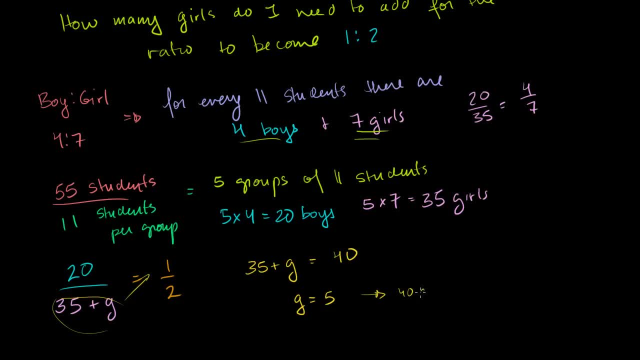 have 40 girls and you have 20 boys And your ratio is 20 to 40,, which is 2 to 4,, which is the same thing as 1 to 2. And we've done our problem. 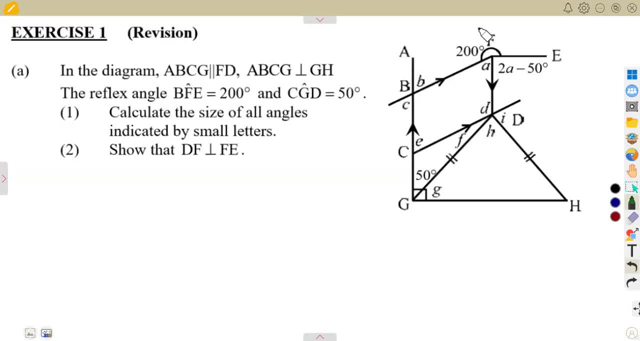 So this is a continuation that we are going to have from the previous case that we had, the introduction, where we talked about all the theorems, the properties of your shapes, the properties of parallel lines. So, on this exercise, which is exercise one, we are given A. In the diagram, ABCG is parallel to FD. So this line, ABCG, is parallel to FD, as we can see from the diagram. 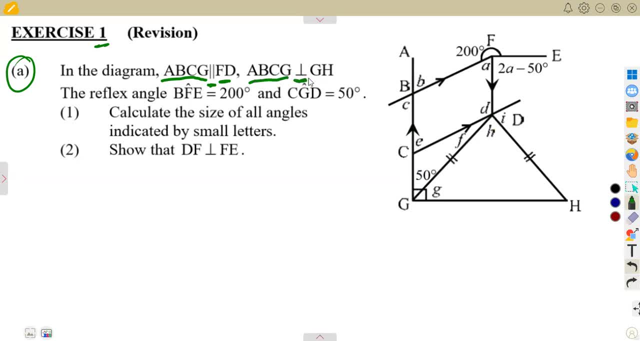 And also ABCG is perpendicular to GH. This time, this line that we are seeing and this line of GH. They are perpendicular, meaning to say they meet at 90 degrees. Also, another part that you are not given: there is this part of the BF and also the line of the CD.